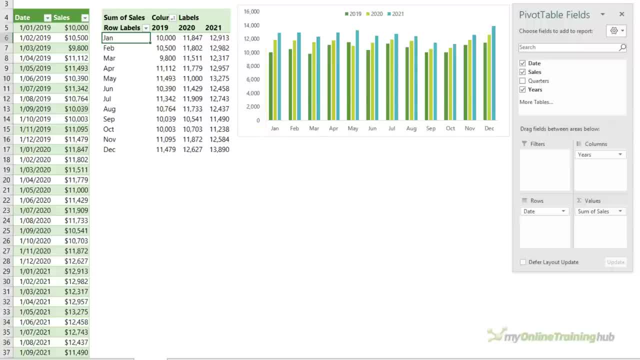 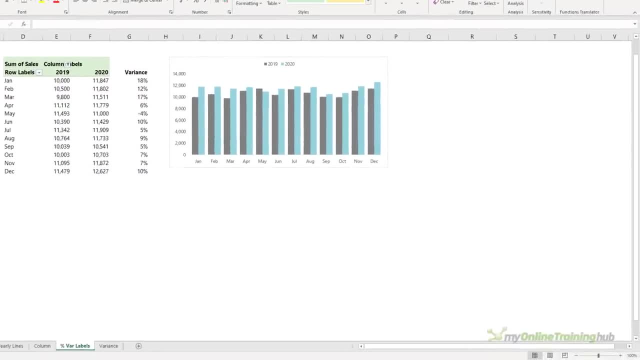 so starting the axis above zero can exaggerate the variances between the columns and mislead our audience. Another option is to show the variance year-on-year, but this only works well for two years worth of data. We can enhance charts like this with some simple formatting. 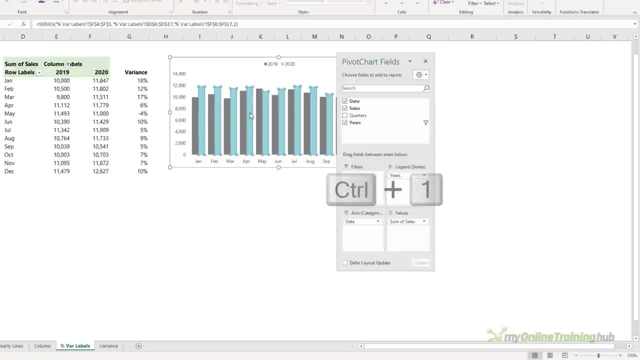 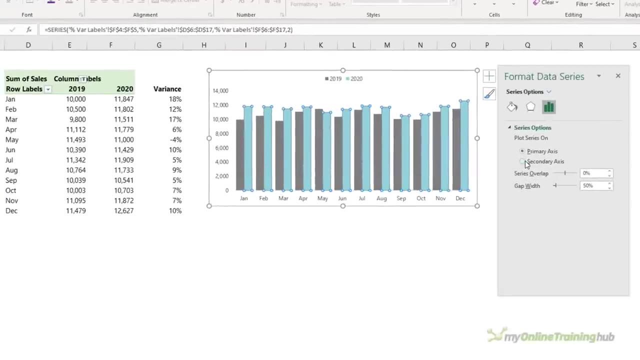 for example, if I select one of the bars, control one, to open the formatting, let me close that pane and I'll bring this over closer to the chart here. if I put one of the series on the secondary axis, I can set the series overlap to 100 percent and make the gap width say three. 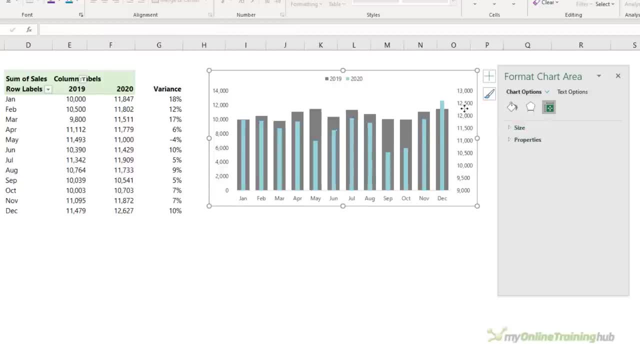 hundred and ten percent. we need to make sure that the vertical axes are on the same scale, and we can see here that they're not, so let's fix that. so this one, the maximum is going to be 14 000 in line with the left hand axis, and now that I've done that, I can hide this. 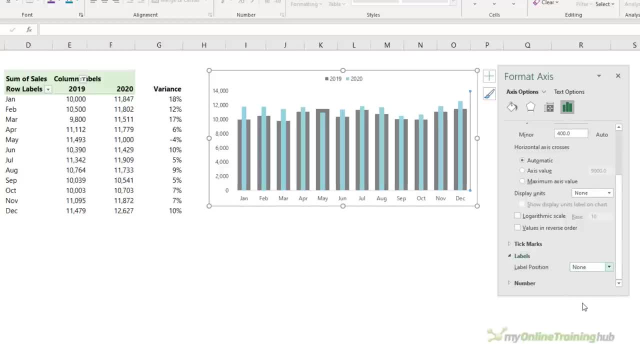 axis. I don't actually need to see it, so let's set it to none. we can also add labels to call out the percentage change. now, in column g, I've inserted a formula, so this chart isn't a pivot chart, it's just a regular chart, and that's going to enable me to reference these cells in my data. 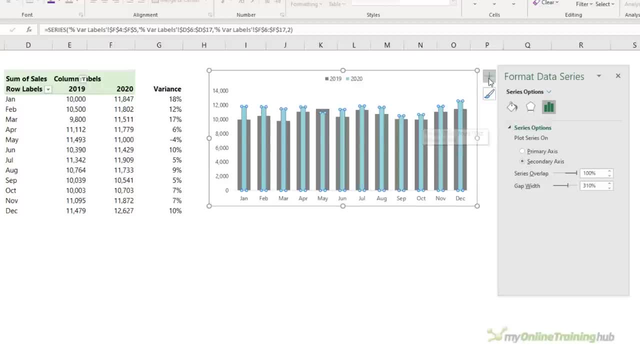 labels. so I want to add data labels to the 2020 series. so let's go into more options. and here, on the label options, I want to deselect the value and instead I'm going to use value from cells and select these cells with the variance that I've calculated. let's set them to blue color. 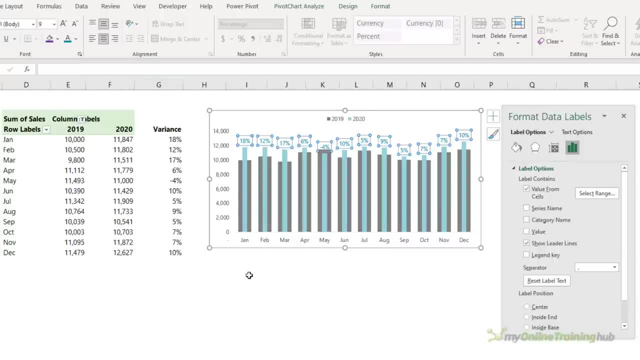 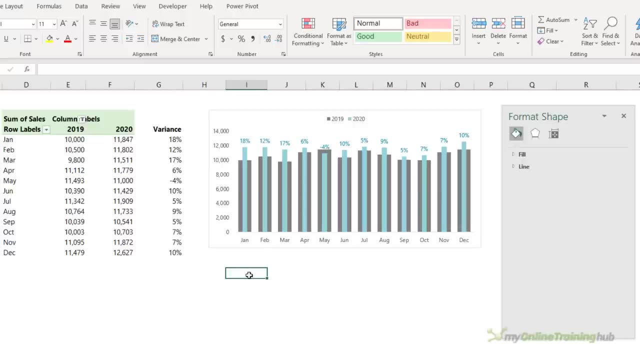 I'm going to go with a slightly darker shade to the column just because I don't want a little bit of a, because font often is hard to read if it's in a pale color and you can't really tell that. it's that much different. Making the labels blue helps. 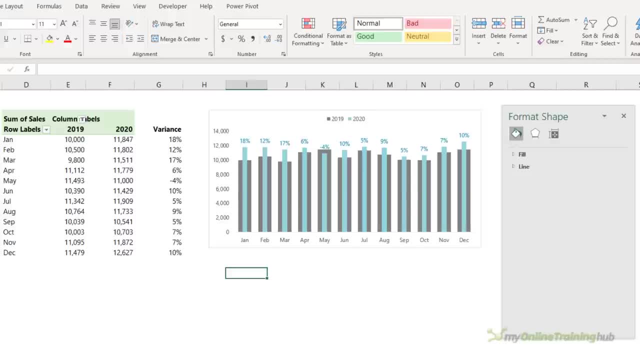 the reader associate those labels with the blue columns. I'm also going to insert a text box for the percentage change legend. Remember, this isn't part of the chart, so I'm going to set that to the same blue color and let's reduce the font size so it's in line with the other legend items. I'm just going to select. 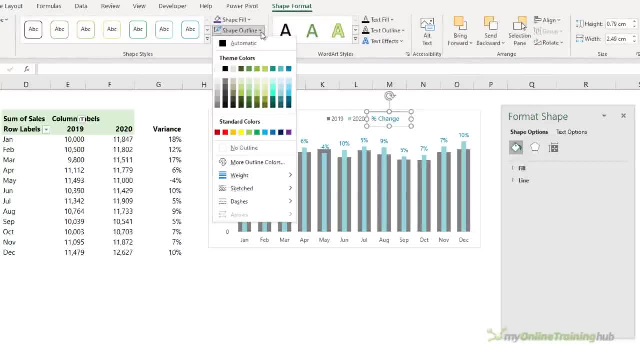 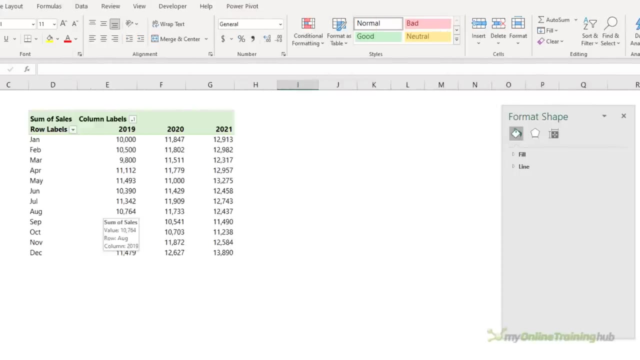 the outer edge of the text box and then remove the outline so that it looks like it's part of the legend. I can maybe move it a little bit closer. So that's one option to highlight the variances year-on-year. Let's look at another. If you want to focus just on the variants, then another. 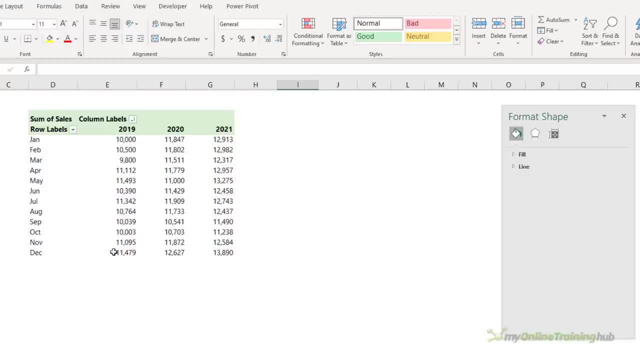 option is to plot the change year-on-year and we can do this in a pivot table. If we look at the field list, you can see I'm just showing the sales data in my file value area, but I can change what's displayed by right-clicking show values. 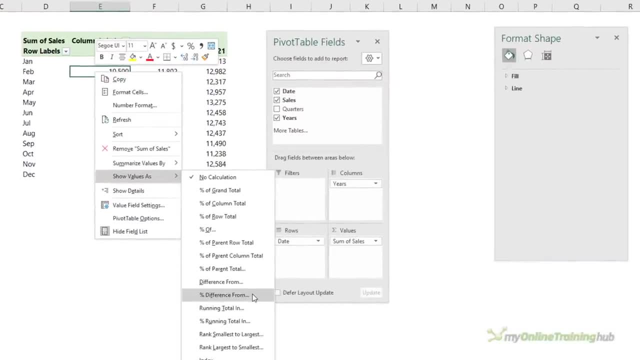 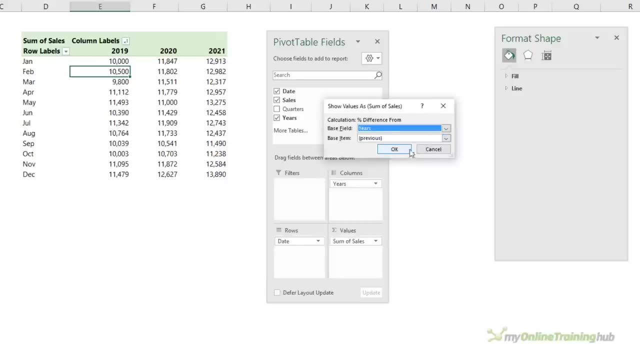 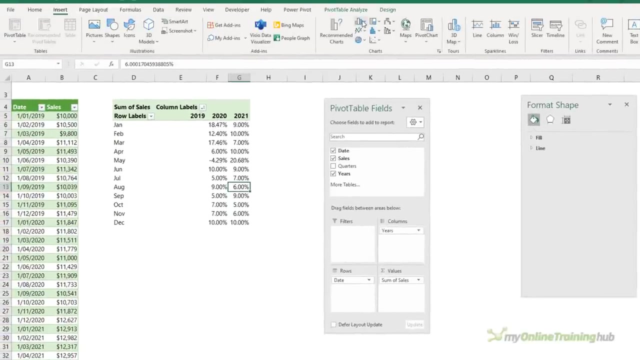 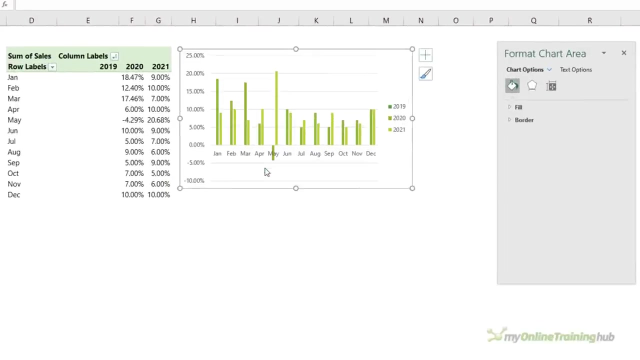 as: and then I want percentage difference from here. I want the base field to be the years and the base item is the previous year. and now I have the percentage change year-on-year and I can plot that in a chart. so let's insert a column chart, place that down. let's remove the fill buttons. I'll do a little. 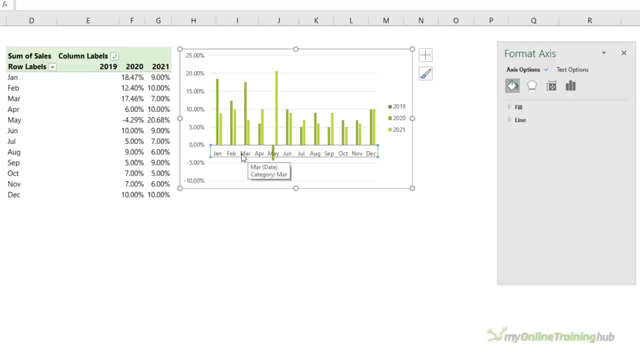 bit of formatting. the first thing I want to do is move this axis so that it's down, so that it sits at the bottom of the chart. so in the labels I want to set it low. I'm also going to hide my vertical axis because instead of having 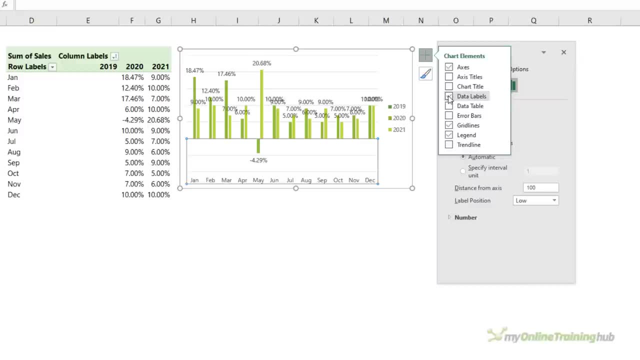 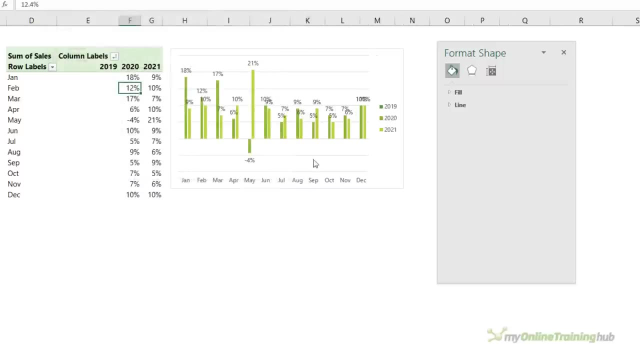 the axis. I'm going to add data labels just for the percentages, and let's format this number. and let's format this number so that it has no decimal places, and that will just make the labels a bit cleaner as well. now a little bit more tidying up to do. let's reduce the gap. 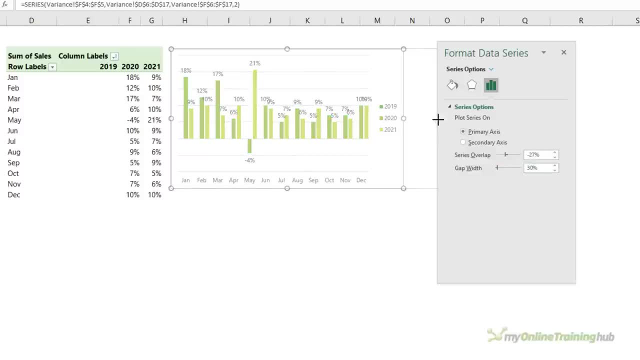 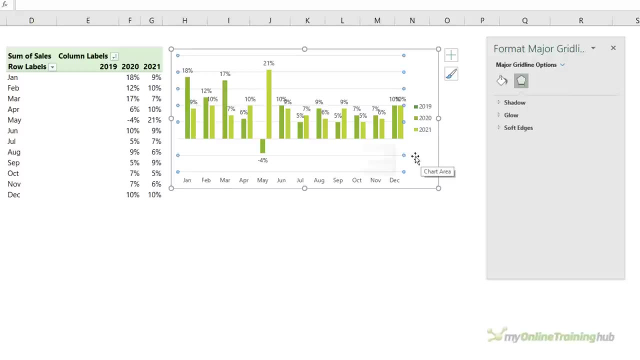 width to say 30%. that'll make the columns wider. we can make the chart a bit bigger. I'll get rid of the grid lines because we don't need them. we have the labels. tells us the exact percentage difference. now you might need to move some of the labels so that they're not overlapping. 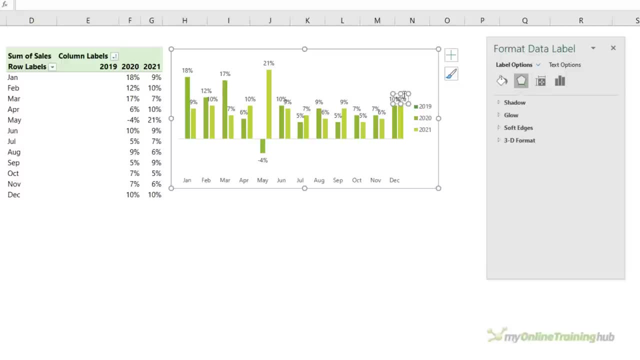 one another. so just left-click twice to select the one you want, and then holding down shift will keep it aligned vertically while you drag it up. let's do the same for this one here, and the others aren't too bad. we could make the columns a bit wider or make the chart a bit wider. that just gives us a.